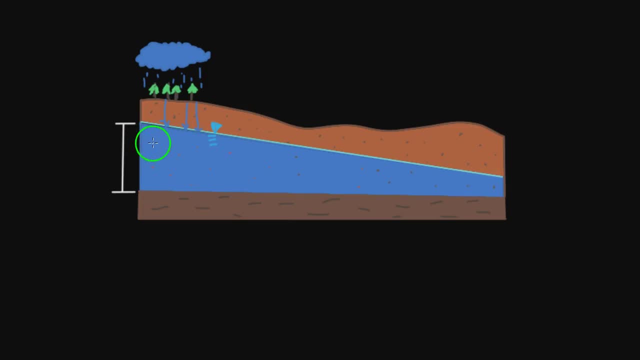 table and it's sloping right, And so you can probably guess which direction this water is going to move. in the aquifer It can't move down right Because down we have our confining layer. It's not going to transmit water, And I'm sure you can guess that it's going to move this way. 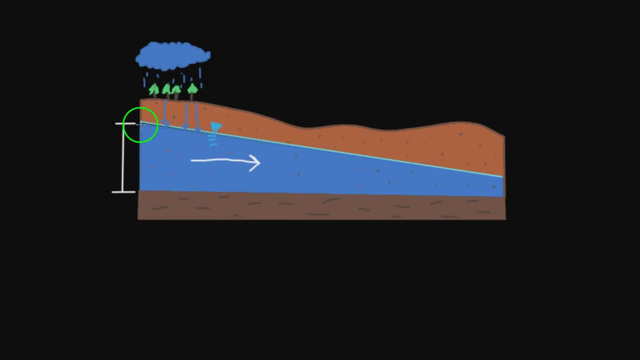 right. But why is that? Well, it's because we have a hydraulic head differential between this point here and this point down here. So it's about right there. So that differential in hydraulic head will move the water from the area of the higher head to the lower head. okay, That's how hydraulic head 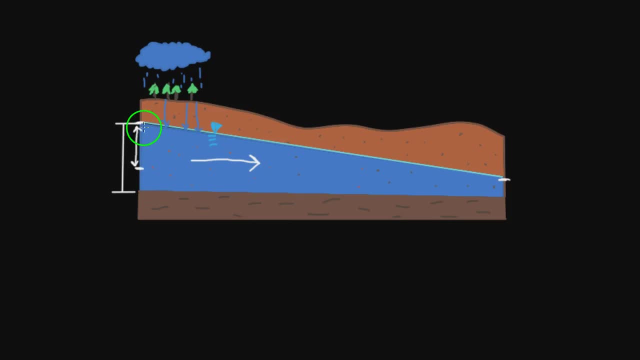 works And you can watch the video on hydraulic heading groundwater to kind of understand more about hydraulic head. All right, and so that's what a hydraulic gradient is Basically: just a difference in hydraulic head between two points And the point with a higher hydraulic head will. 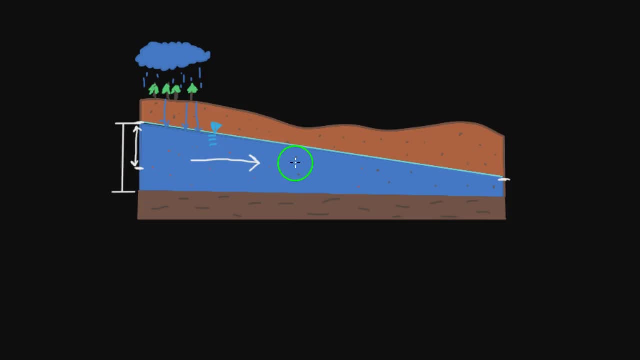 force water to the lower hydraulic head. okay, Pretty basic, pretty simple, but important concept to know and understand. Okay, so now let's look at a potentiometric surface map- And we're going to use this example here- this side view of the aquifer, and we're going to look at it on a 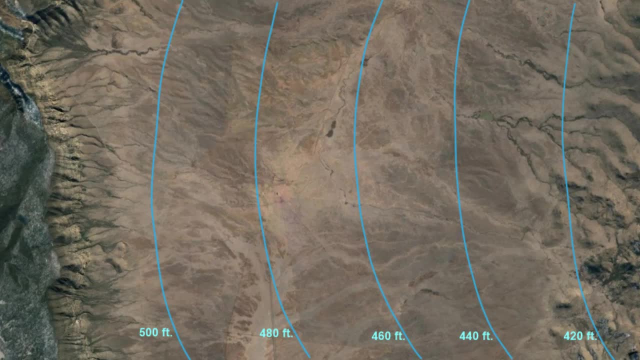 potentiometric surface map. So let's look at this example where we're looking at the side view of the aquifer, And let's look at it from the top, so like a map view, And so you'll see here's the land surface and here's our little. 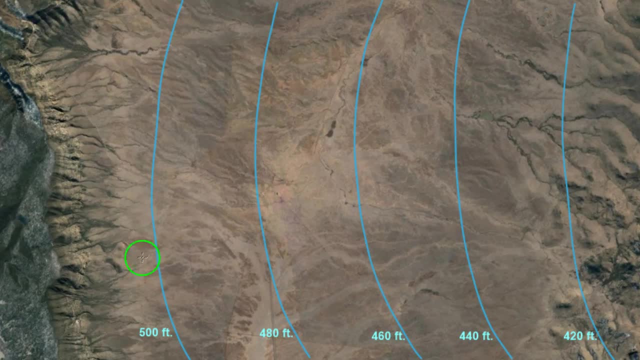 highland area where we're getting our precipitation coming in and recharging the aquifer. And you'll see, we have these blue lines on the map And these blue lines are called equipotential lines And these lines represent the elevation of the water in that aquifer or the hydraulic potential of the. 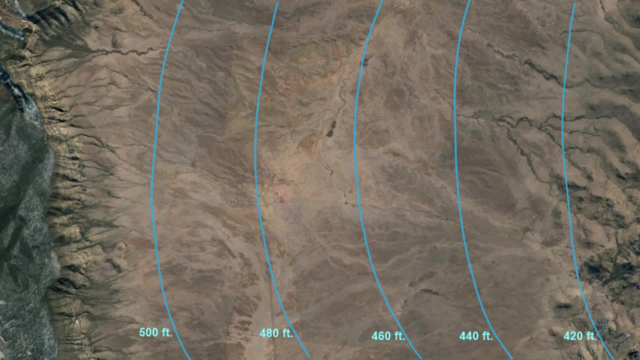 water in that aquifer above a specified datum. And you remember, we measure hydraulic head in units of length, so these are units of length or elevation here. okay, And so here we have a 500 foot equipotential line, And so the water in the 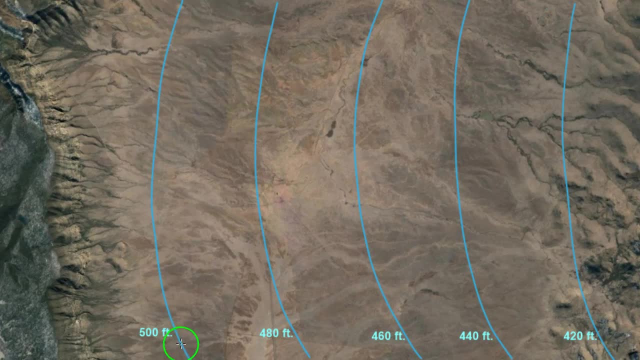 aquifer along this line has a hydraulic head elevation of 500 feet or a hydraulic potential of 500 feet above sea level. So we have a 20 foot contour interval between these lines And you can kind of think of this as a topographic map in a way, but instead of 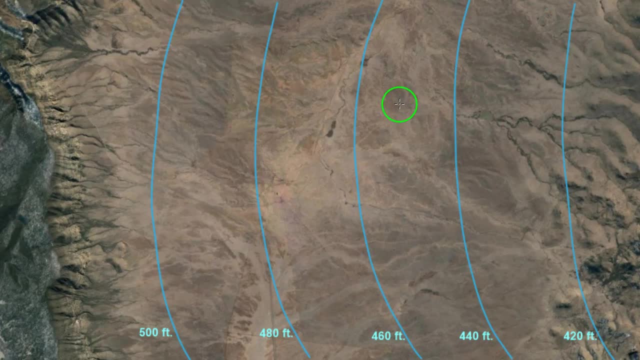 representing the land surface. it's representing the hydraulic head potential of the water in the aquifer. okay, And so in an unconfined aquifer, these lines represent the actual water table right, Because the water in the aquifer is not under pressure like it is in a confined aquifer. 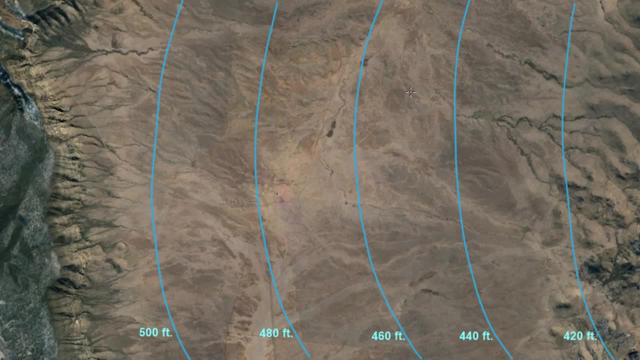 In a confined aquifer, these lines would represent the hydraulic head potential of the water in the aquifer. okay, And if that doesn't make sense to you, watch the unconfined versus confined aquifer video that I have. I'll put it in the comments section below. 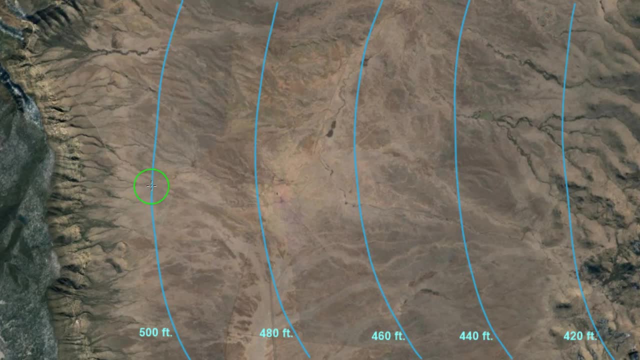 Anyway, remembering that we're going to be doing a lot of work on this. so if you're interested in water flows from areas of higher hydraulic head to lower hydraulic head, you can see that the water in this aquifer is going to flow to the right because it's going from an area of higher. 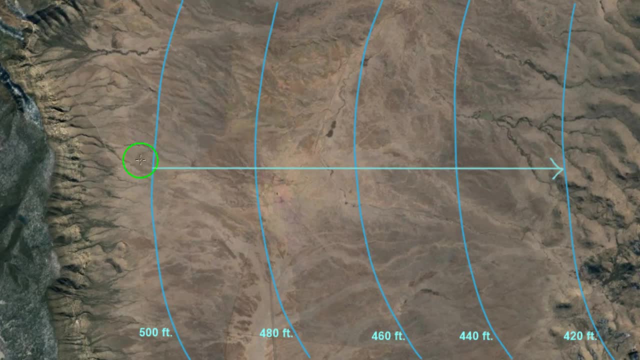 hydraulic head potential to lower head potential, And that's how water moves in the earth. okay, And when you're looking at a potentiometric surface map such as this, you can always figure out which way the water will travel by drawing a line perpendicular to these equipotential lines. 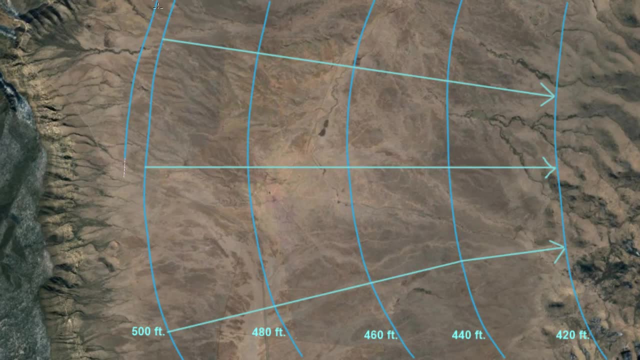 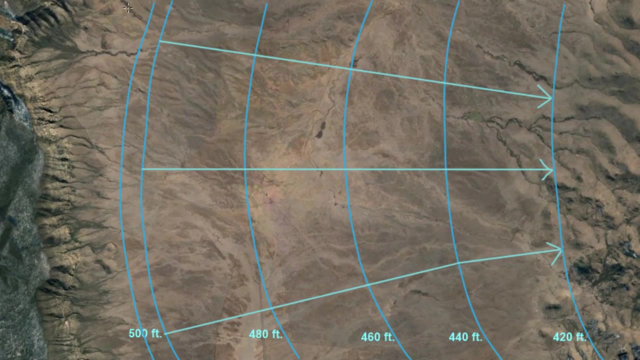 Okay, let me illustrate one other point here. So say, we had lines, equipotential lines, that were really close together, like this- Oops, didn't want to do that, Like, so What would that represent? So this is the 500 line here, and this would be 520, 540. 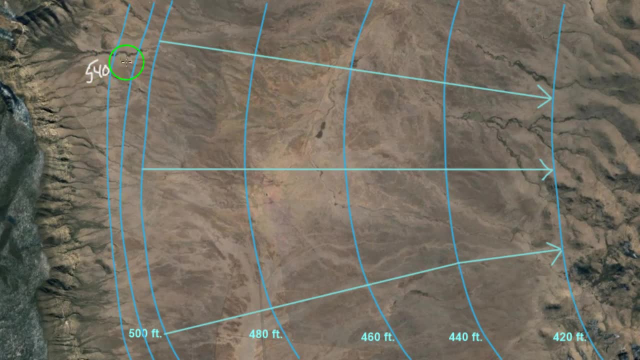 So let me just label that really quick: So 540, and then 500 here. okay, So water is still going to travel the same way right From higher to lower. But what does this represent when we have lines really close to each other? 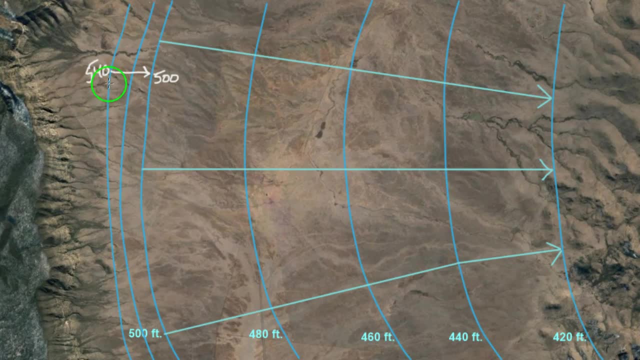 like that. Well, kind of like how I said earlier about how these equipotential lines sort of act like a topographic map for hydraulic head of the water within the aquifer. As you may know, on a topographic map when you have lines that are very closely spaced like this, 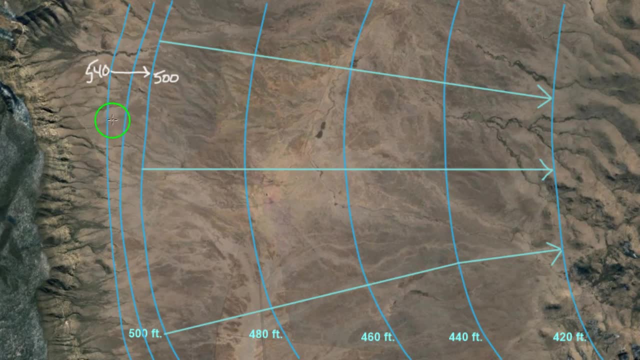 that will mean a really steep slope, right, Because you have this large elevation change over a very short distance compared to this distance. So it's the same thing with a potentiometric map like this. So from here to here would be a very steep hydraulic gradient, and then from here 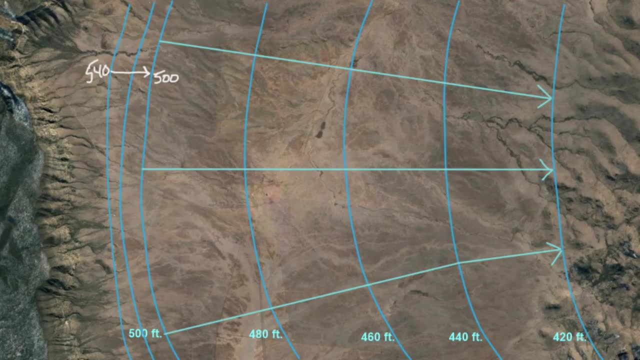 to here would be a more mellow hydraulic gradient. okay, And these maps are very useful to geologists and engineers and anyone trying to figure out where the water is moving within the aquifer. So you may ask: how can we know the elevation of the water table? 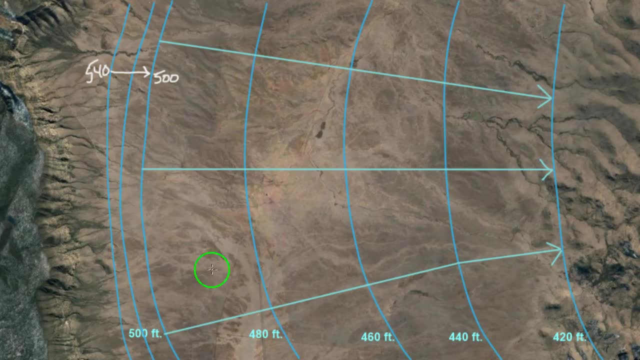 and draw these equipotential lines, And the answer to that is that we have to measure the water table in wells constructed in that aquifer. okay, So let's say we have a well here that we may measure and a well here and maybe a well like right here that we measured. okay, And so yes, 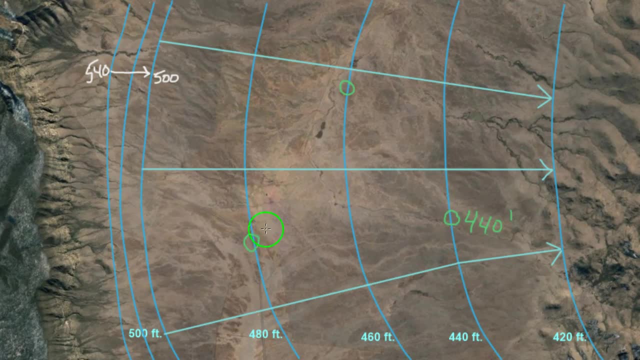 we measured this one at 440,, 440 feet above sea level. We measured this one at 480, and then this one at 460.. And so, based on these data, we can start drawing these equipotential lines. Let's say we have another- well, maybe like right here, and we measure that to be 490, okay. 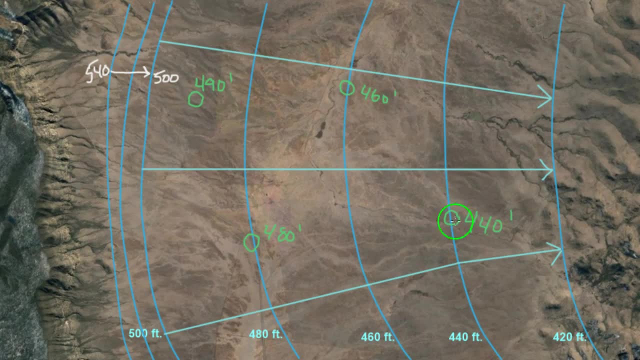 So, based on these data, we can start drawing these equipotential lines. okay, We know the water elevation right here is 480,. we know right here it's 440.. We've measured over laterally to kind of draw these lines to fit our data. So measure 460 there, we can kind of draw that line there. 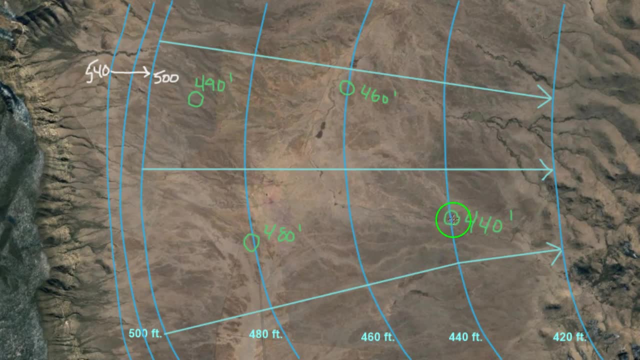 and then wrap it in between these two, because we know we're at 440 here and 480 here, right? So it has to fall somewhere in between. there We're drawing the lines based on the data that we have, on the data that we've collected from our wells. okay, that about does it for this video, if you have. 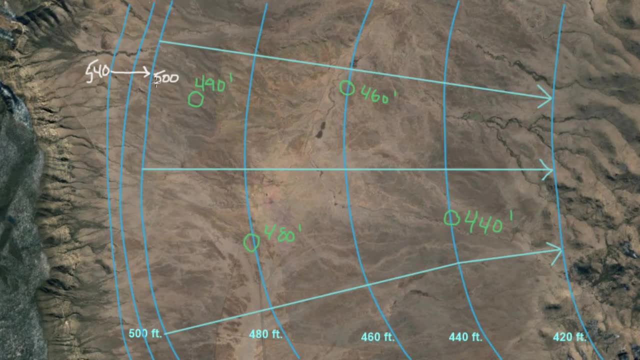 any questions, leave them in the comments. like the video, subscribe to the channel and we'll see in the next one.